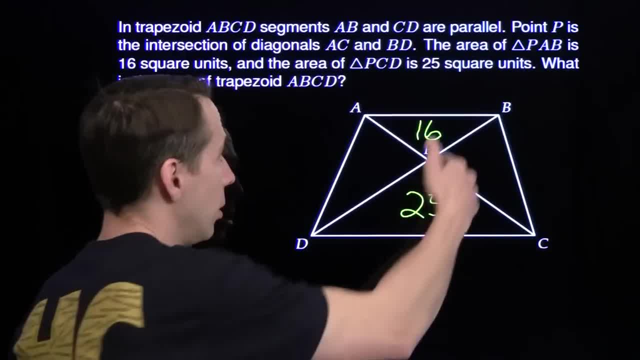 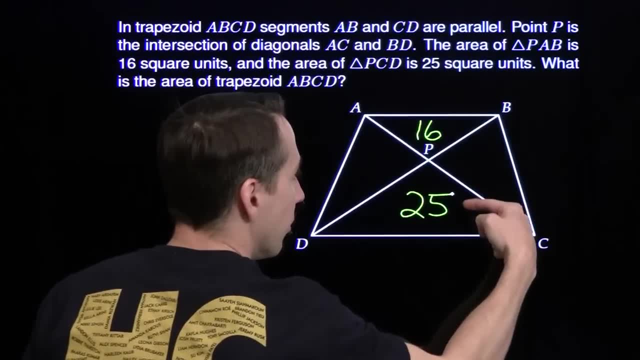 have their areas. so we know the ratio of their sides, because, well, the ratio of the areas of two similar triangles is just the square root, OK, of the ratio of corresponding sides. So ratio of the areas is 16 to 25.. That means the ratio. 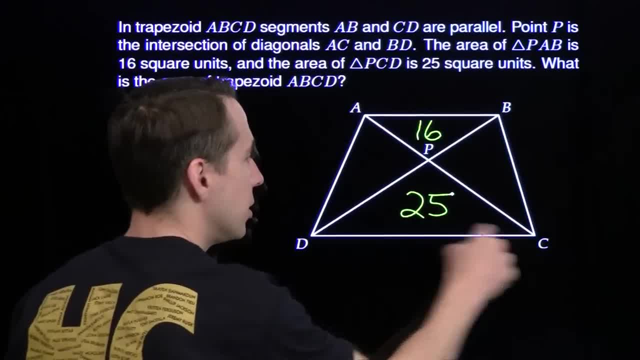 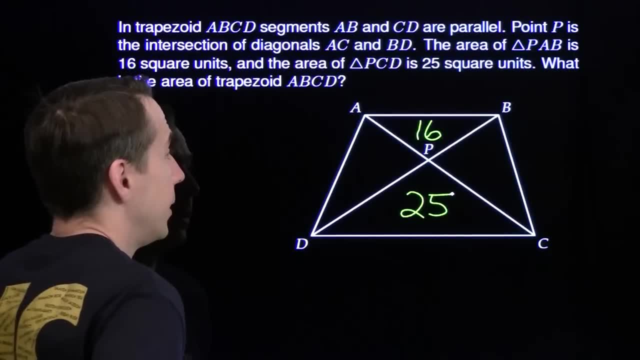 of corresponding sides is 4 to 5.. So this to this is 4 to 5.. This to this is 4 to 5.. This to this is 4 to 5.. How's that going to help? It's time for one of my favorite geometry. 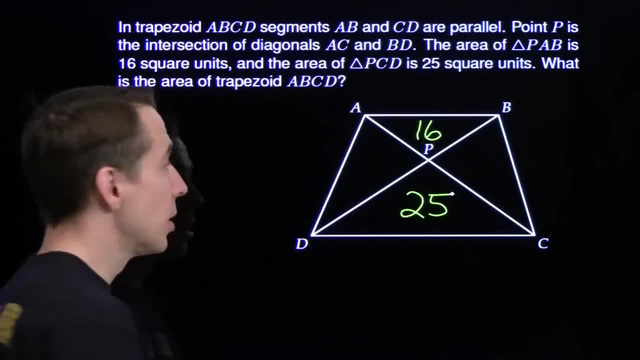 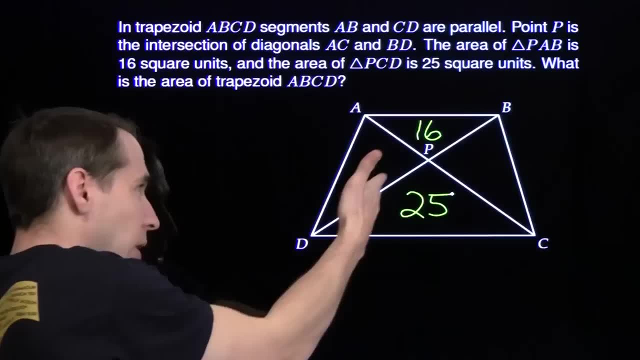 problem-solving strategies. right here We have a problem about areas. We have a couple of triangles right here that have sides- BP and PD- that are along the same line. Now check this out. Let's look at the areas of these two triangles. They share an altitude. 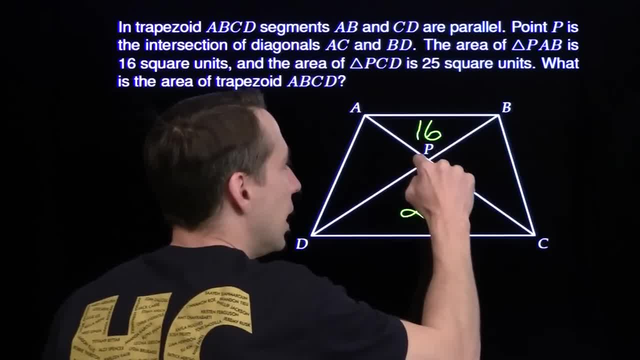 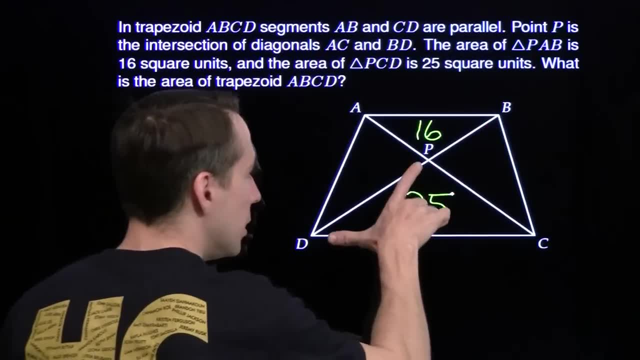 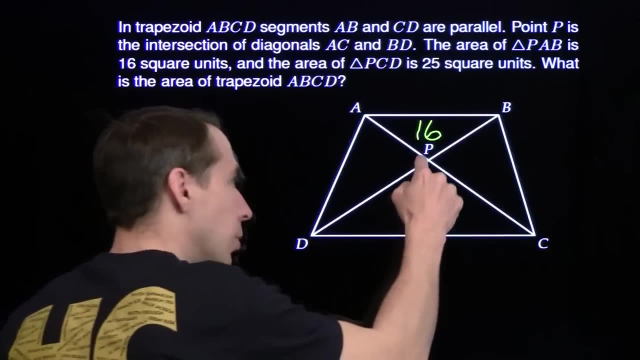 from A, And that means that the ratio of the area of this triangle to the area of this triangle is the ratio of this base to this base, Because to get the areas of these two triangles we're just going to multiply this base by that altitude and then divide by 2,. 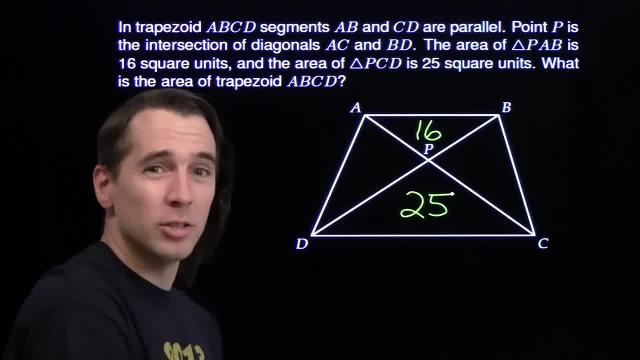 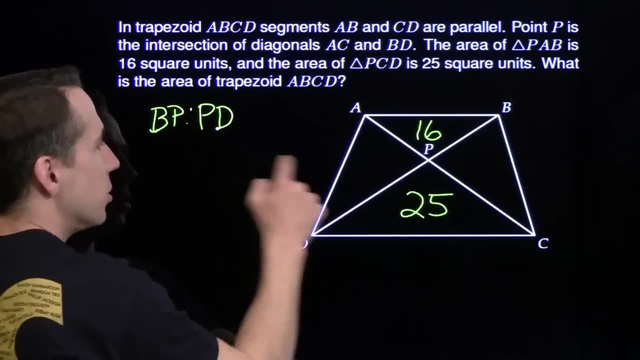 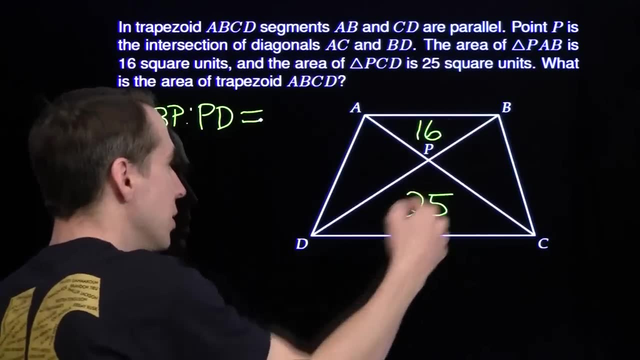 multiply this by 2.. We have the same altitude. So the ratio of the areas is just the ratio of these two bases, And we know what this ratio is. We figured that out already from our similar triangles. Ratio of corresponding sides of these two triangles is 4 to 5.. So now we know the ratio. 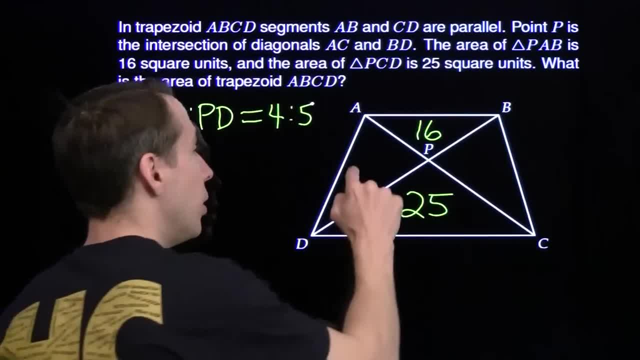 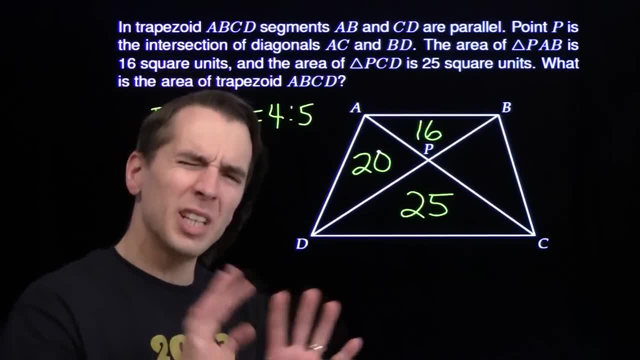 of this area to this area is 4 to 5, which means this has area 20.. We do the same thing over here. We got a strategy that works once in a problem but doesn't quite finish it. Run that back. 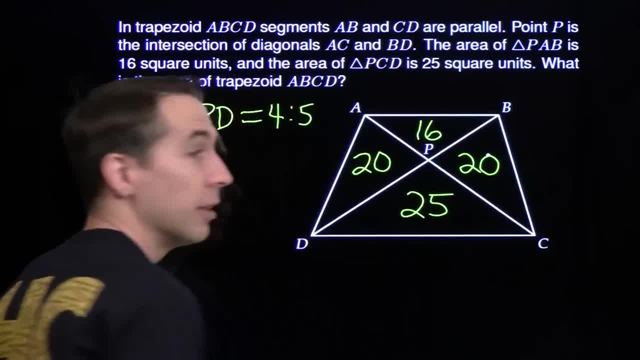 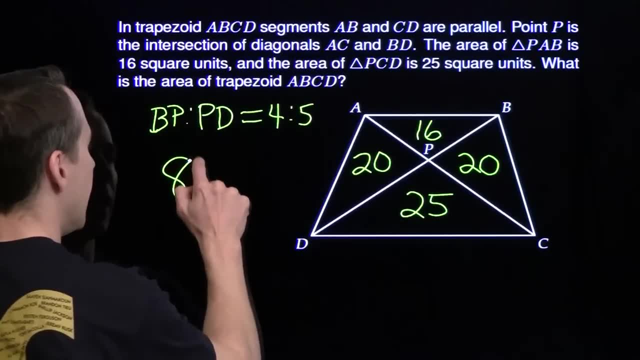 Do it again. We do it again over here. The area of that is 20 as well. So now we've got the area of the trapezoid. 16 plus 25 is 41.. Add on the two 20s and we get 81.. 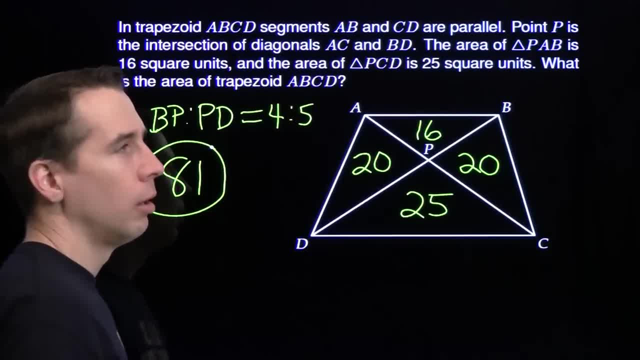 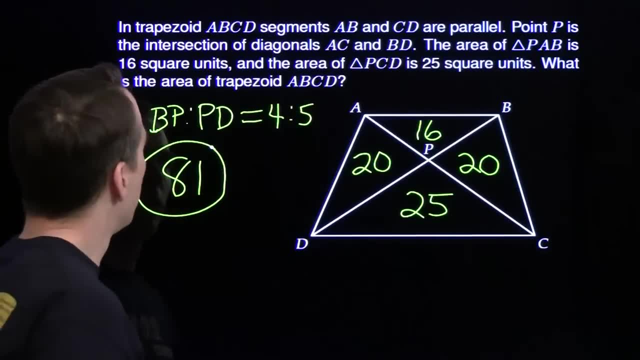 We're finished with What? Oh, you had that a long time ago. What? It's just 4 plus 5, and then you square it. What? Yeah, 81 is 9 squared. So Oh, Wait a second. If 6 plus 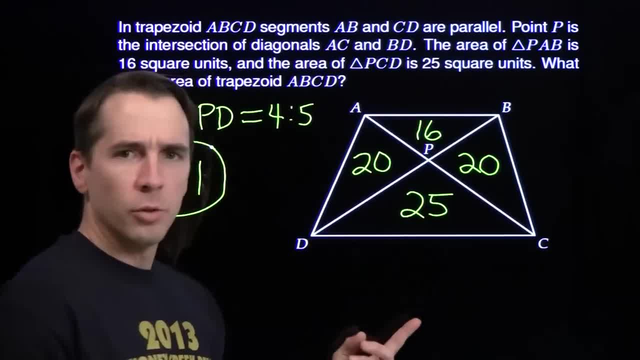 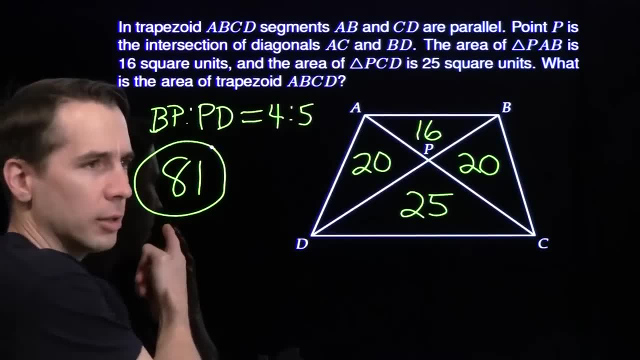 5 is 16 up here. that's 4 squared. 25 here is 5 squared. And you're telling me that you then just take the 4 and 5, add them and then square it and you get the Well it. 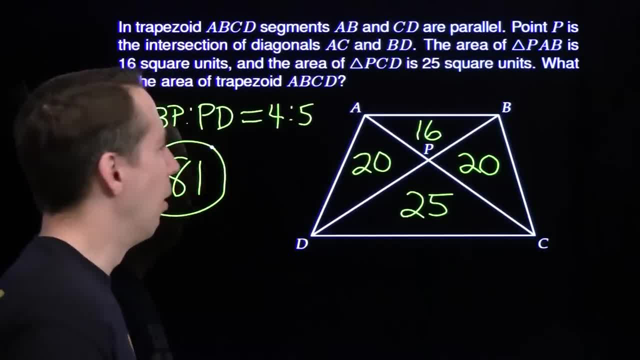 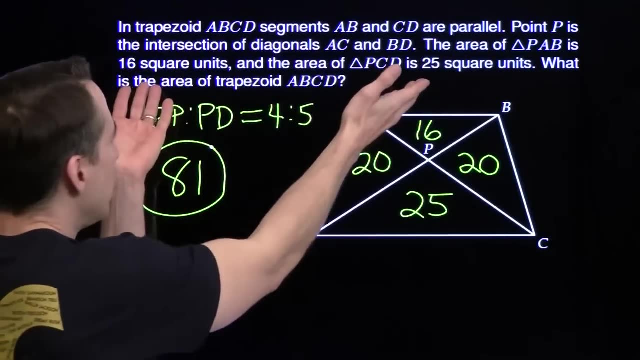 works here. That always works. No, No, Okay, Oh, that's, Wait a second, I'm going to give you a little homework, all right. Harvey's telling me that in this problem. he just looked and he said: okay, this is 4 squared, this is 5 squared. and then he just adds 4 and 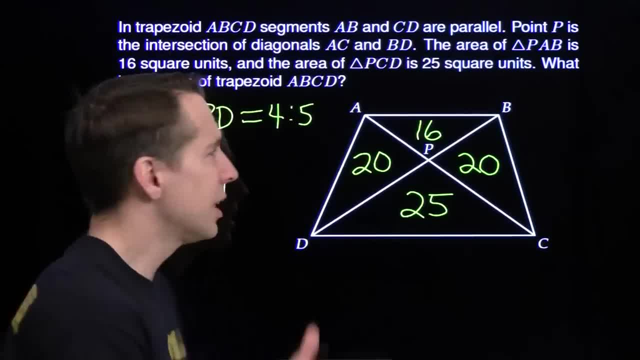 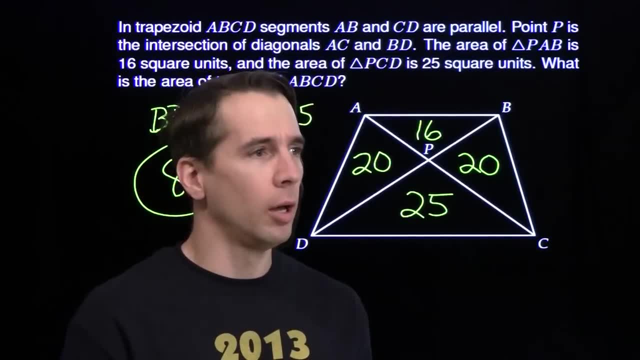 5 and squares it and gets the right answer. And it does get the right answer. but he's telling me that would work. whatever these two numbers are, I'm not sure I'd buy it. So here's your homework: Try to prove Harvey wrong. What? Oh nobody proves Harvey wrong. 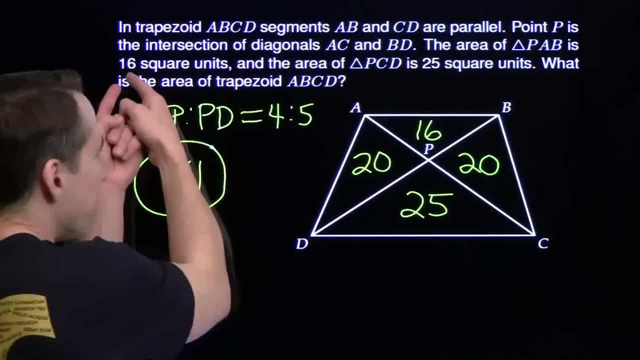 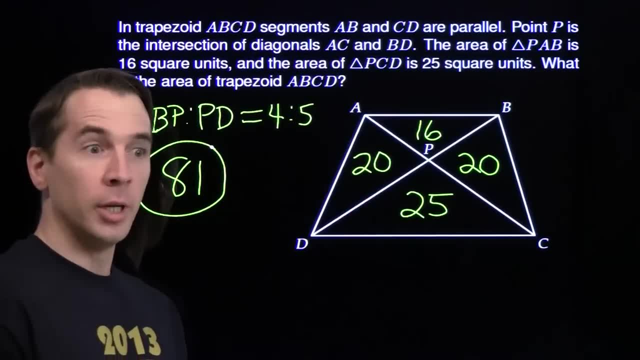 All right, Try to prove that Harvey's right. All right, Prove that if you start with any two numbers here and here, any two positive numbers, you take the square root of this one, square root of that one, add those two results and then square your sum and you'll. 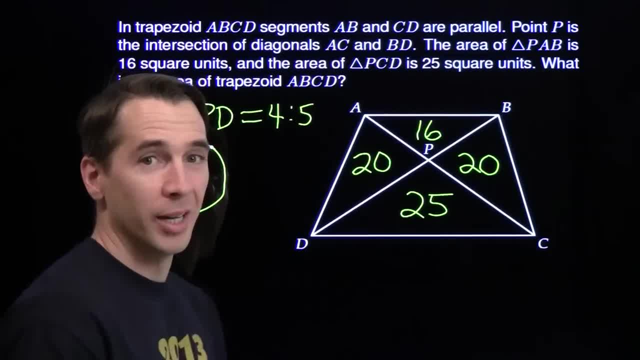 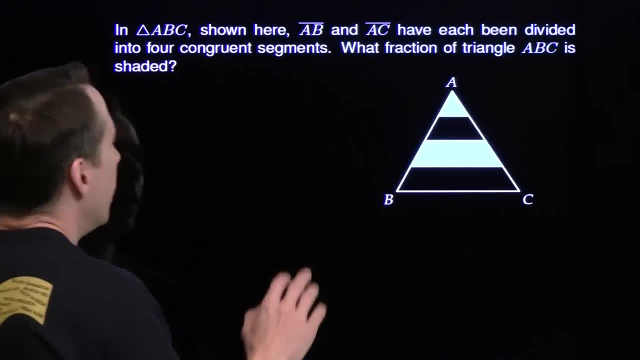 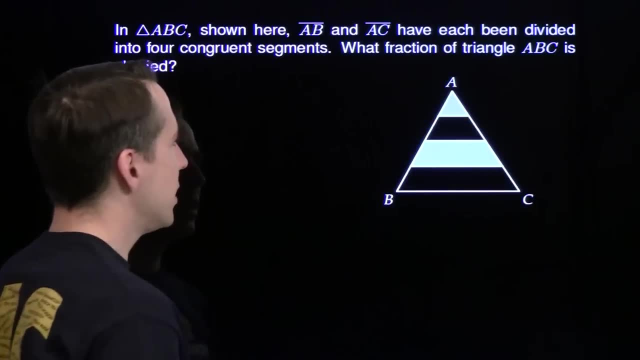 get the answer. I'm a little suspicious of that, but Harvey's usually right. But oh, yeah, yeah, Okay, Whatever, We're going on to the second problem. Here we go. That looks like Charlie Brown, He's Triangle Man. What do we got here? We got triangle ABC. We divide. 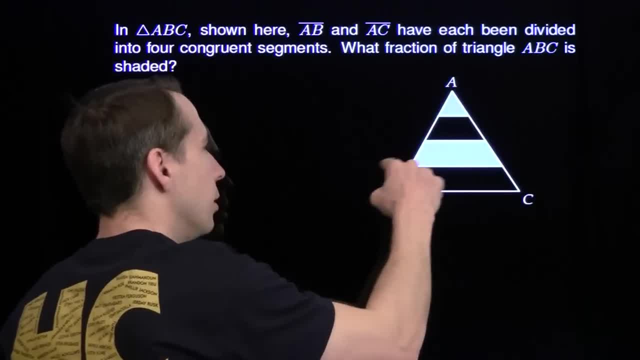 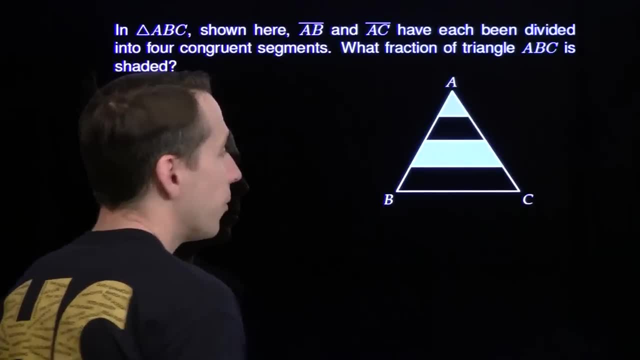 each of these sides into four equal pieces and then draw these little lines and make these little shaded regions. All right, Grab my pen and get to work here. Well, first of all, all of these segments here. these are parallel. We have some similar triangles here. 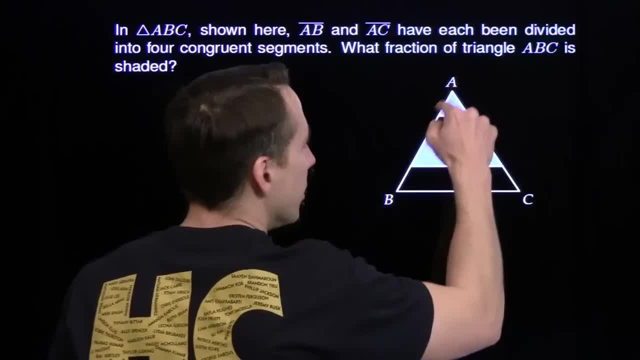 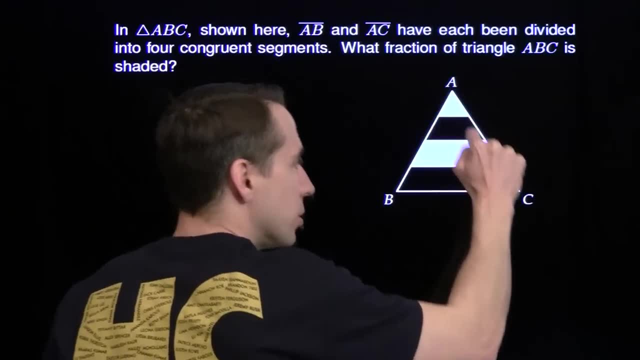 We can see that with a little side angle side similarity here, This is a quarter of this, This is a quarter of this And of course you have the same included angle here. So the little triangle is similar to the large triangle. Of course we can do the same thing. 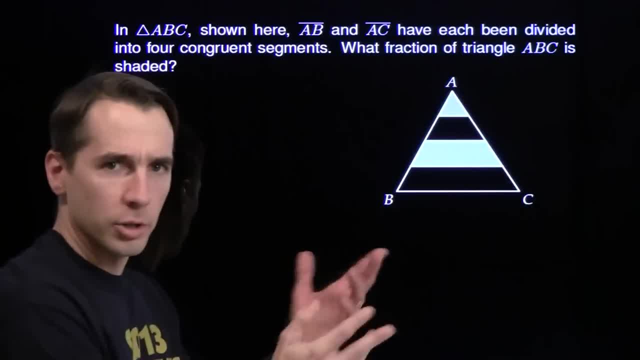 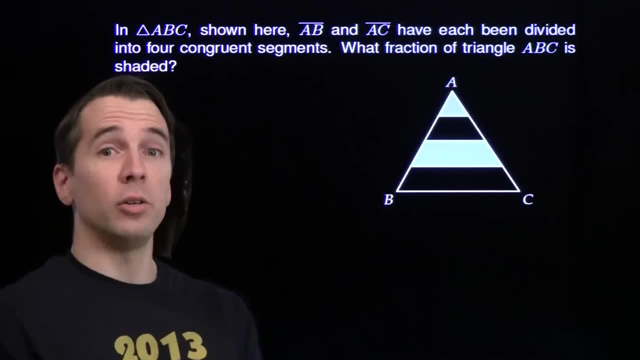 Here. this triangle's similar to a large triangle, this triangle's similar to a larger triangle, and so on. Now, this side length is one quarter of the whole thing. so the area of that itty-bitty triangle is the square of one quarter. It's one-sixth of a quarter. That's what we're. 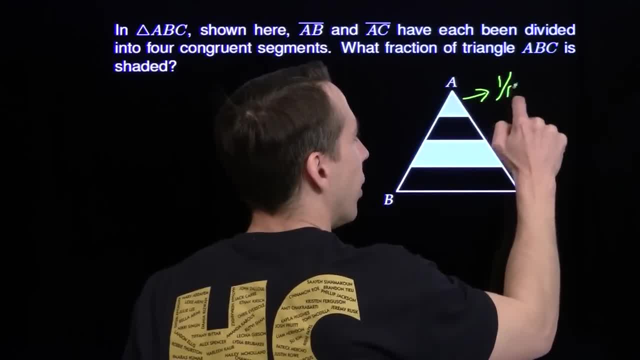 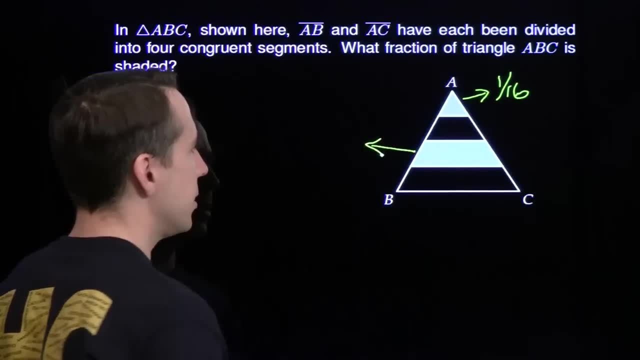 doing, It's the square of one quarter, which is a quarter of a quarter If you divide that. So this little triangle is 1: 16th of the whole thing. But what about this region down here? How are we going to deal with that? 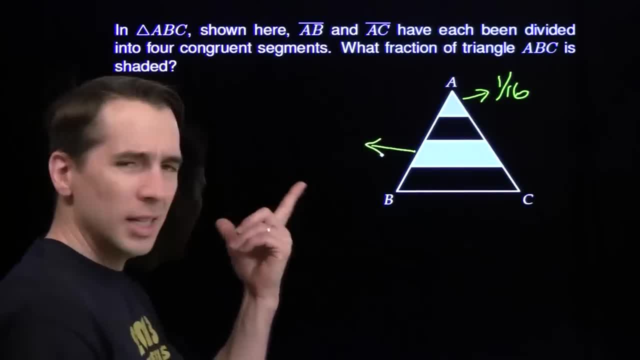 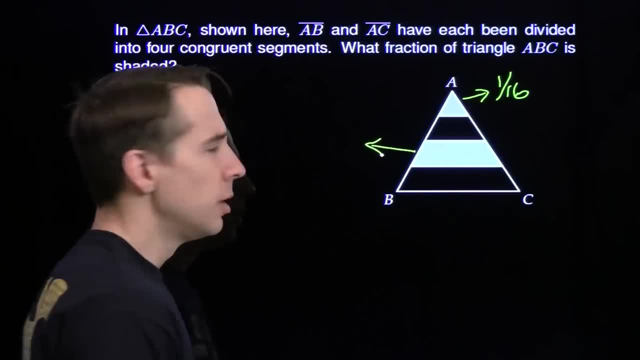 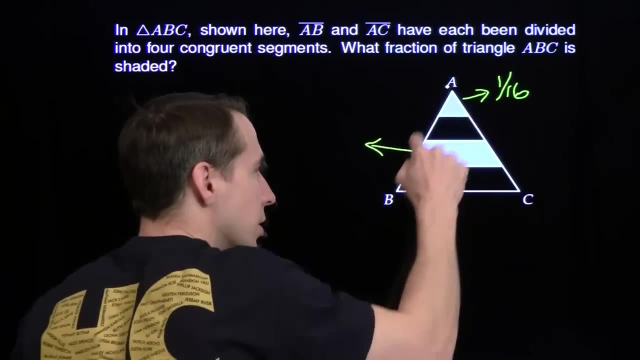 That's not just a triangle, but it is what's left. if you start off with this triangle right here, Cut that triangle out of this bigger triangle. So let's start off by looking at this triangle right here and its side lengths are 3 quarters. 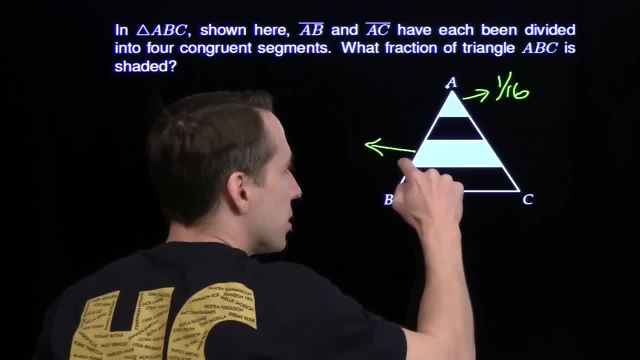 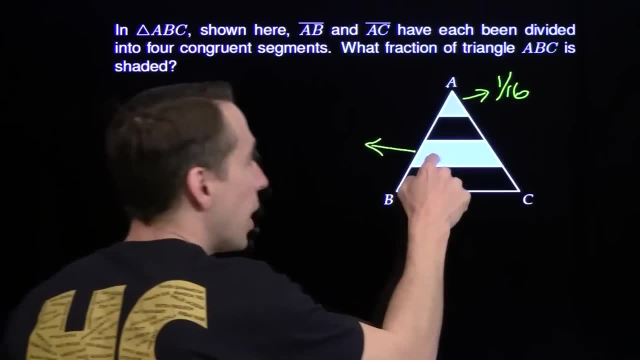 the side lengths of the big triangle. So the area of this big triangle is the square of 3 quarters, is 9, 16ths the whole thing, And then we're going to subtract off to get this region down here. we're going to subtract. 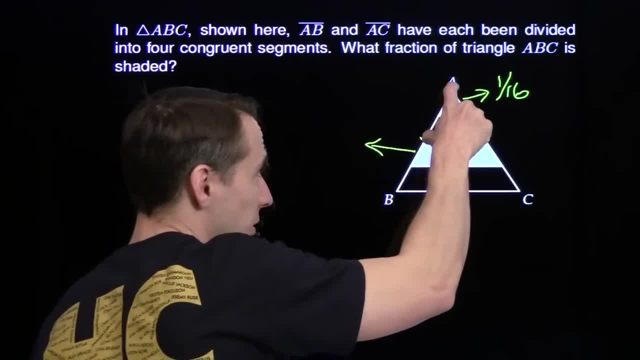 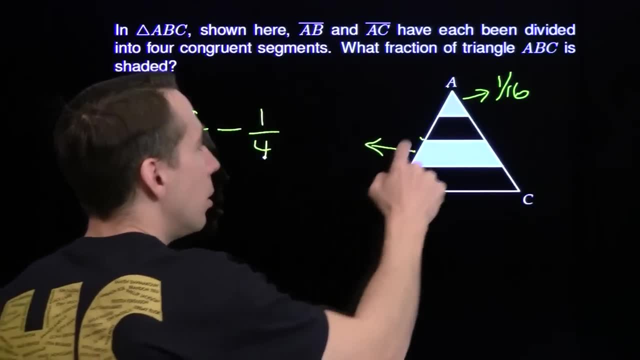 off the area of this triangle And the sides of this triangle are half the sides of a large triangle, So its area is 1 quarter the area of the whole big triangle. So this piece down here we just subtract 9 16ths minus 1 quarter. 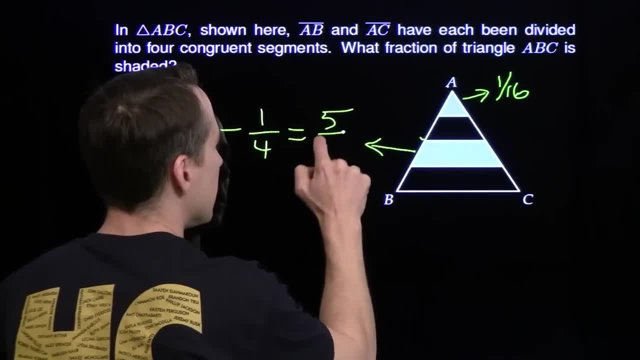 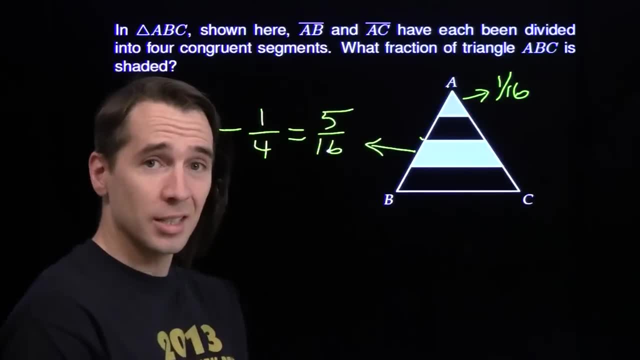 1 quarter is 4.. 4 16ths- That gives us 5 16ths. So we take the 5 16ths of the whole triangle that's here, add it to the 1 16ths of the triangle up there and it gives us 6 16ths. 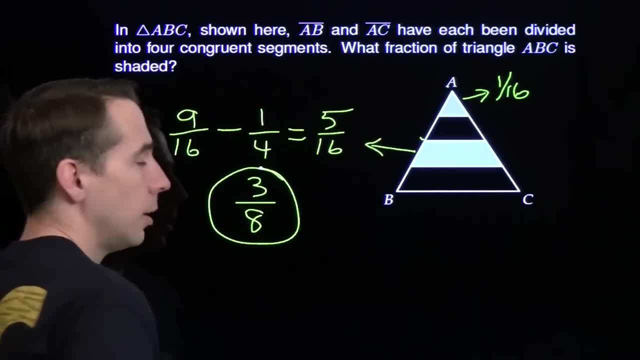 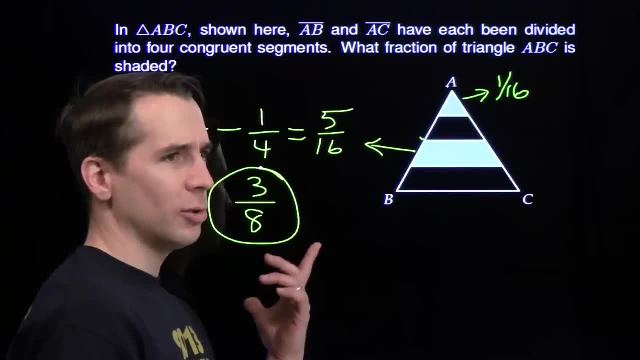 Simplify that and we get 3, 8ths, And so you've got a smart way to do that one. Of course you do. What is it What? 6 little triangles out of 16 little triangles. It's obvious and you're done. 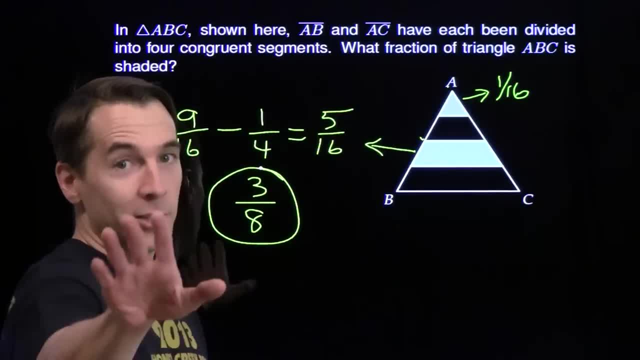 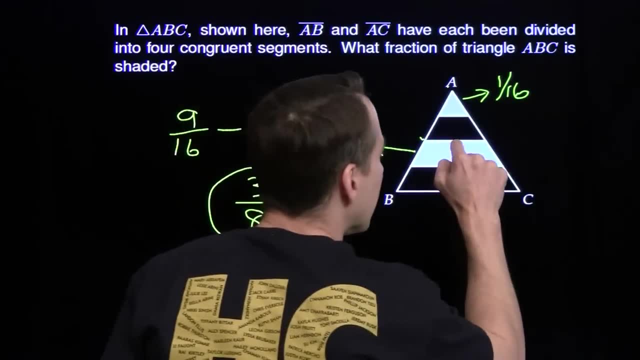 What? Oh, That's really clever. Check this. You're going to like this. I actually understand this one, so check this out. We've got a little triangle up here. Now we can come down here and we can break this into little triangles as well. 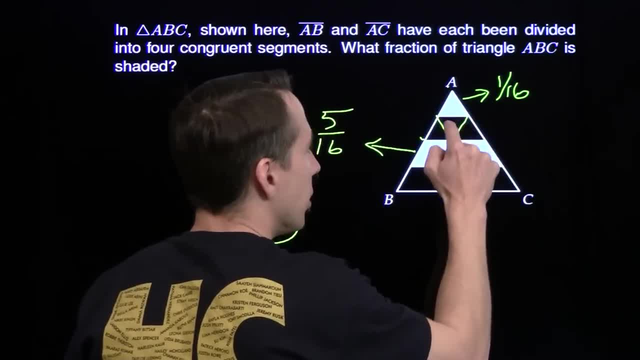 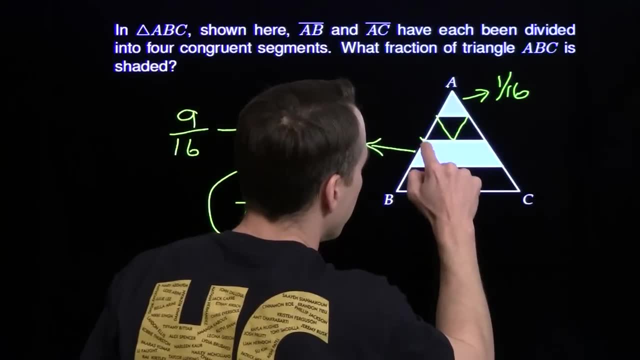 You're going to take the little midpoint down here and go doink, doink. These are midpoints up here. So this splits this triangle into 4 congruent little triangles. Well, now we just take these little triangles and keep going down here. 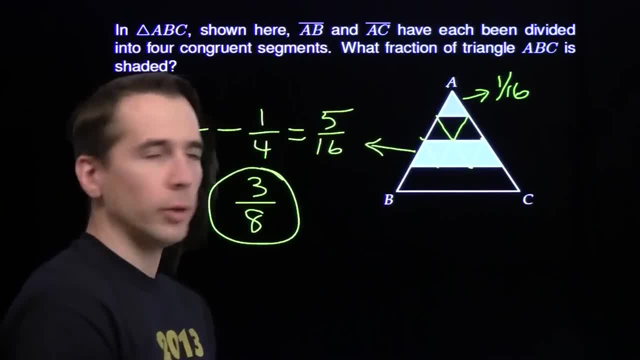 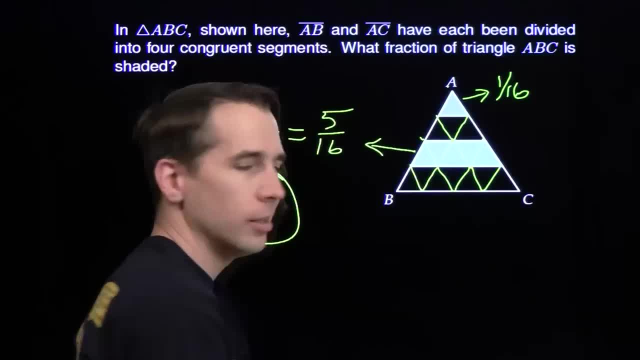 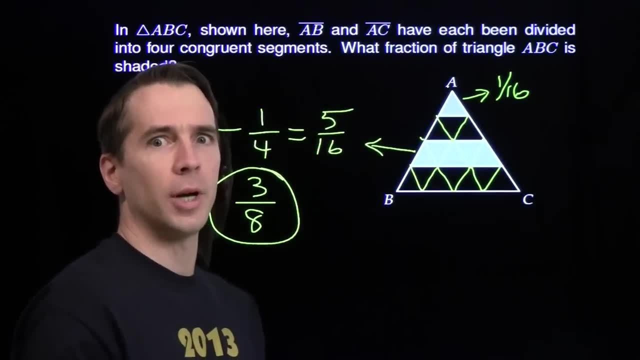 Doink, doink, doink And there we go. Break the whole thing up into 16 little triangles: 1,, 2,, 3,, 4,, 5, 6. We've got 6 of these little triangles out of these 16 congruent triangles. 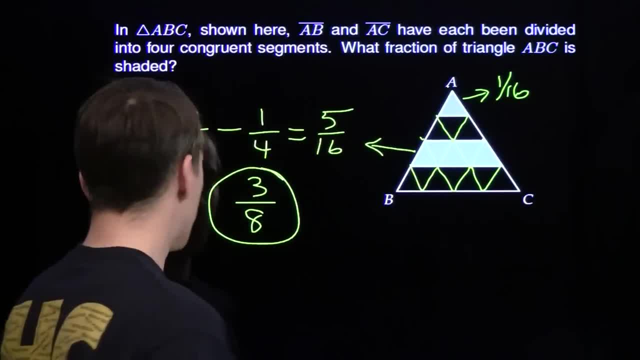 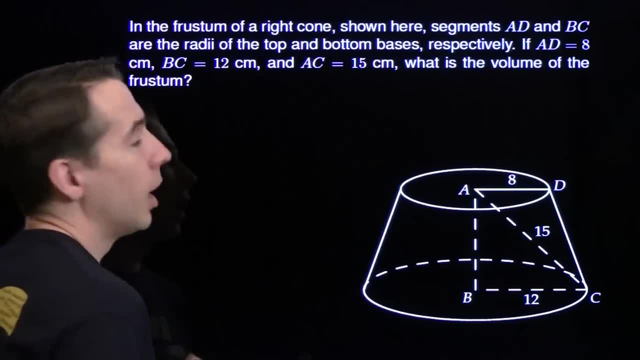 So this shaded region is 6 out of 16.. That's pretty slick, Harvey. This is why we keep you around. All right, Here we go. Last problem, And yes, Harvey, I'm going to tell you right up front: I need some help on this one, because 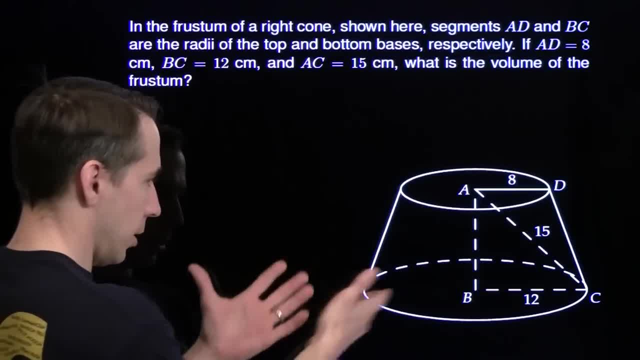 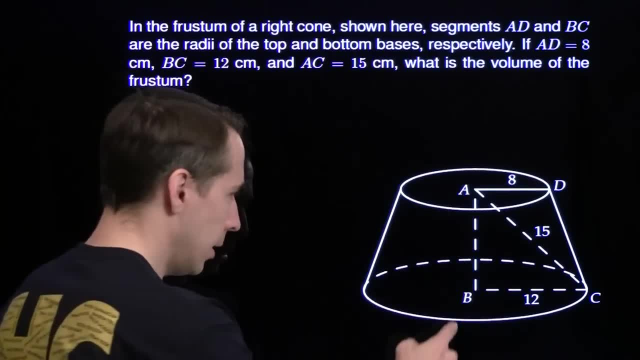 that's scary. What we're starting off here is with a frustum. All right, We start off with a frustum and we're given the radius of the top piece is 8,, radius of the bottom piece is 12, and we're told that this length right here is 15, and we want 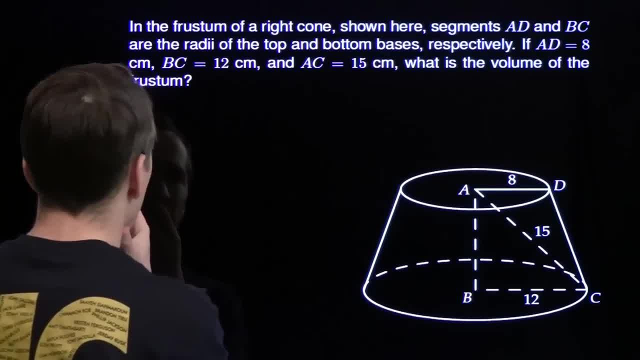 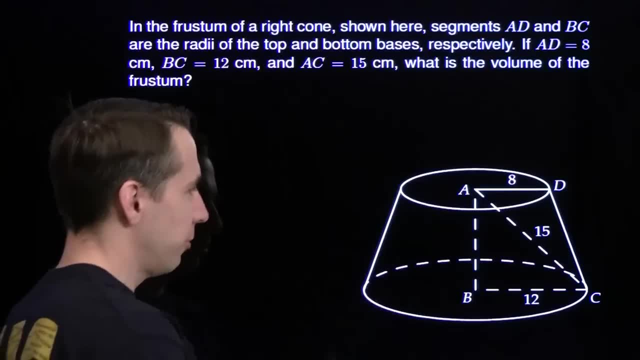 to find the volume of this frustum thing. Now, I know there's this wacky formula- and Harvey probably knows this wacky formula- for finding the volume. What? Oh, you don't need to know the formula because you can just prove it whenever you want it. 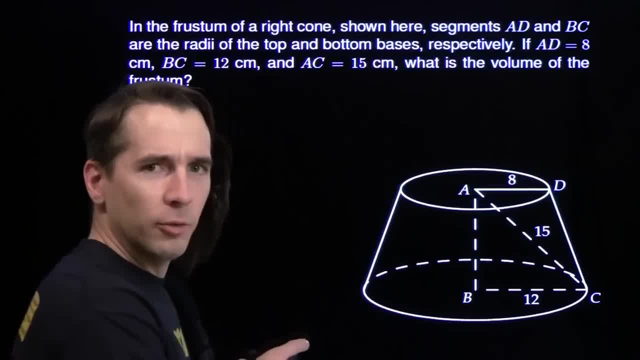 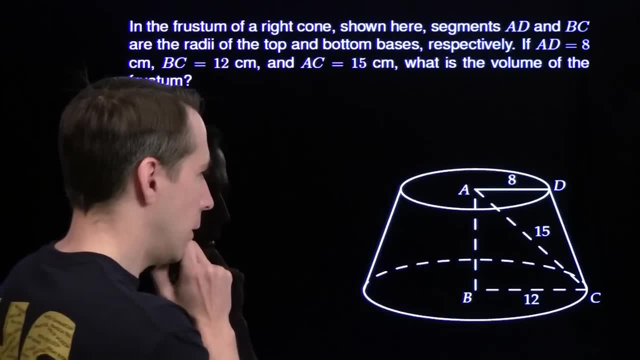 That's great, Harvey. I think there's a wacky formula, but I'm too old to remember those sorts of formulas and things. So what are we going to do? What Use the cones? It's a frustum, Harvey. 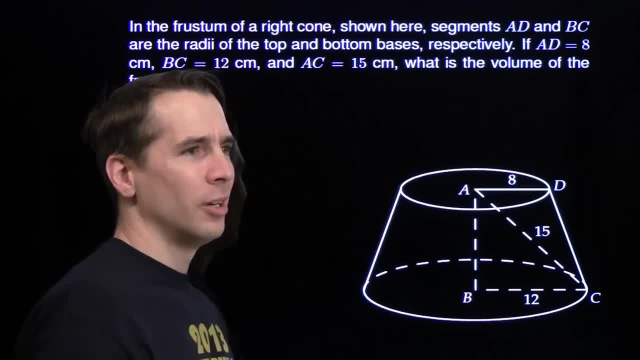 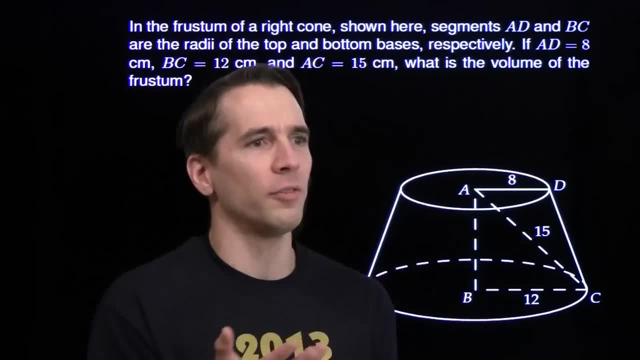 Read the problem. This isn't a cone. Where do you see cones? What's a frustum? Well, Harvey, a frustum is just what you get when you start with a cone and you chop a little cone off the top. Oh, those are the cones. 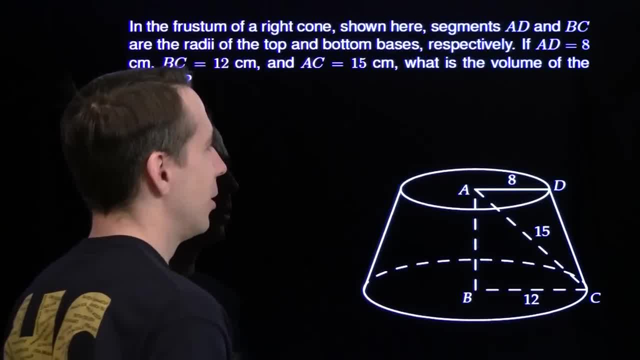 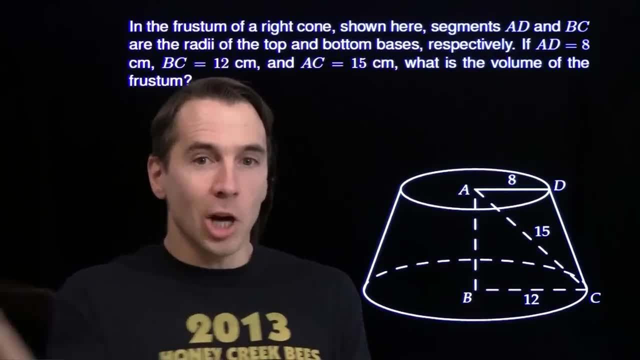 Okay, Harvey, We'll start with the cone. All right, We'll start with the cones. Ah, that's really clever. Check this out. How do you make a frustum? You start with the cone and then you chop a little cone off the top. 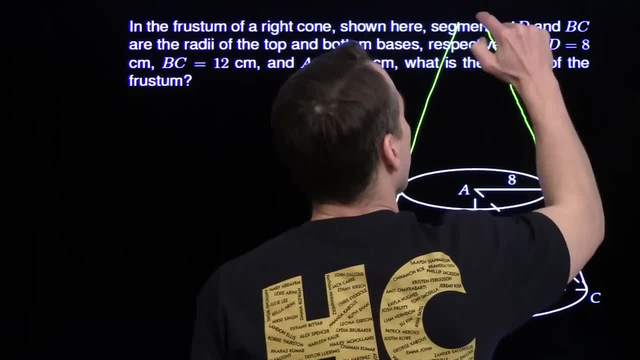 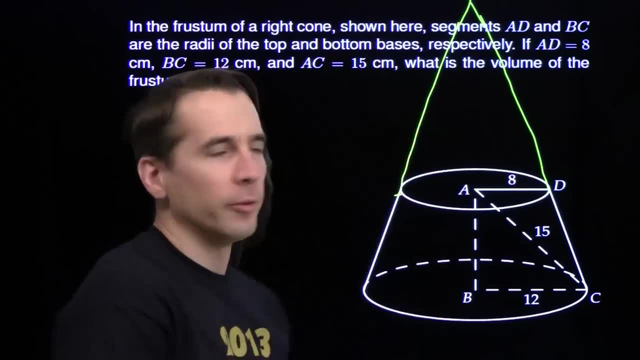 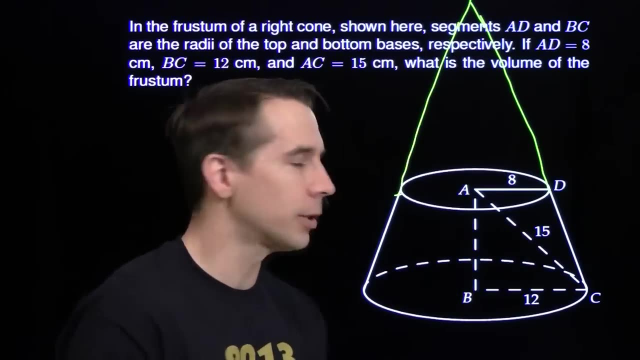 So we're going to start with the cone, Extend this up here and pretend we start off with a huge cone and we chop the top cone off. And how are these- this little cone up here- related to the big cone? The little cone is similar to the big cone. 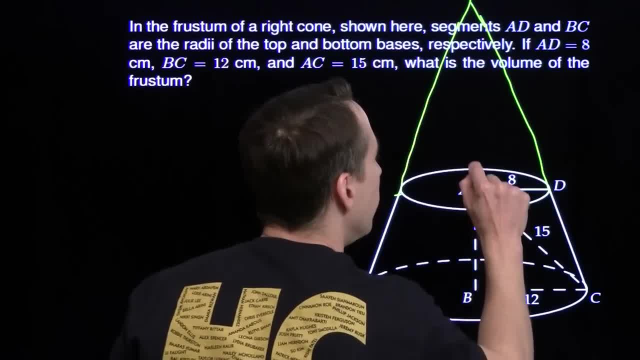 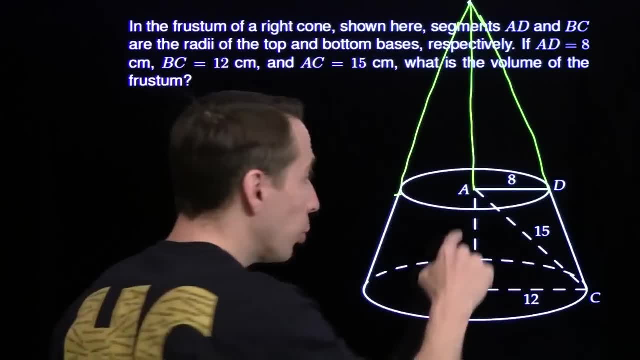 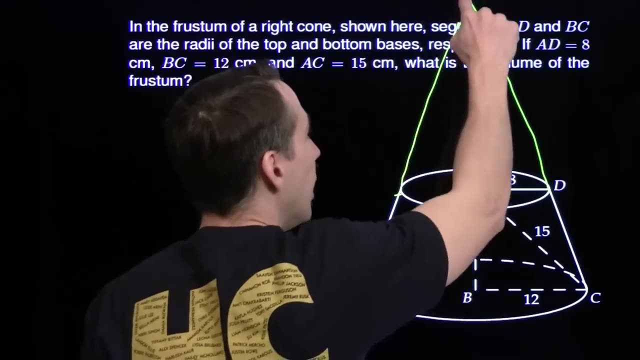 Oh, that's really clever. So we just continue this all the way up and well, we've got similar cones. We also have some similar triangles right here, Parallel lines, similar triangles. we have parallel lines right here: 8, 12.. 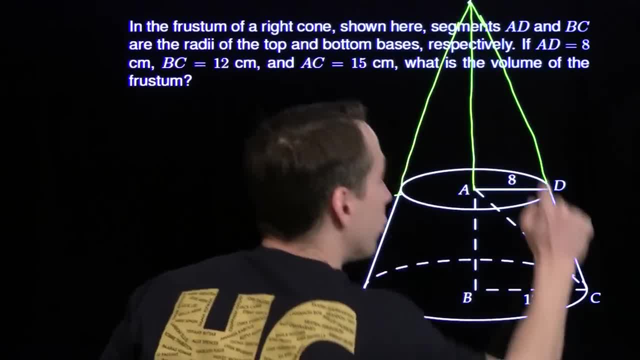 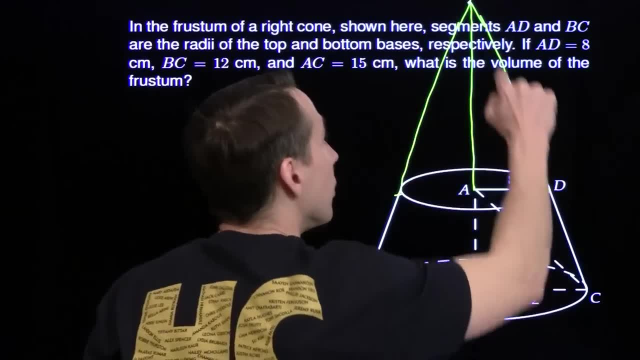 And now we know the ratio of this triangle to the larger triangle. the ratio of the corresponding sides is 8 to 12, is 2 thirds. So now we see that this, the little piece, the piece that we cut off here, It's height is 2 thirds of the whole thing. 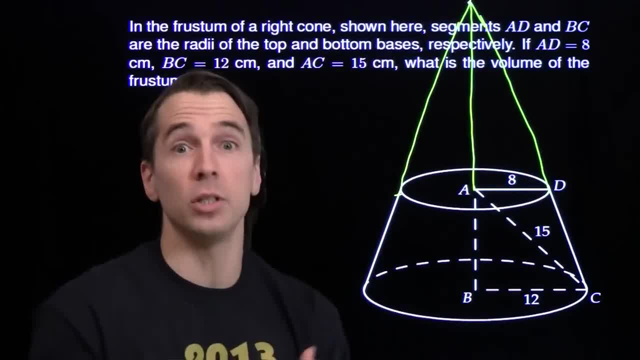 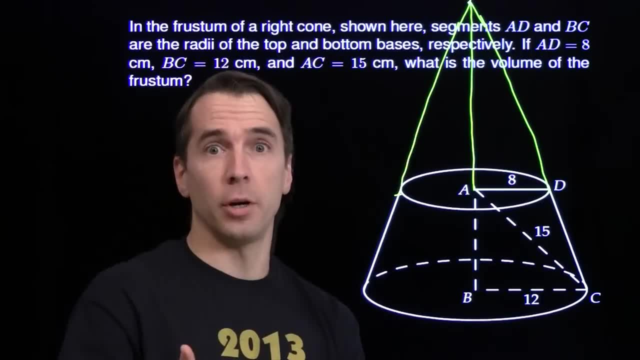 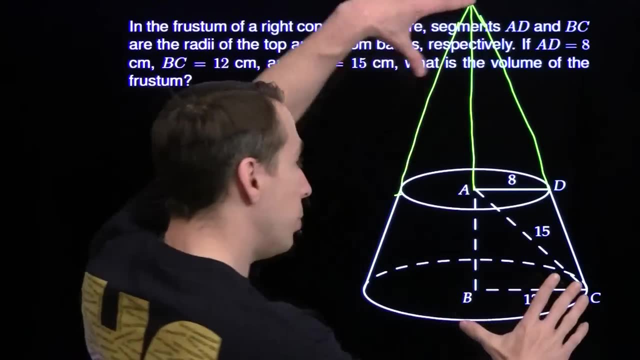 So the ratio of side lengths of our little cone to our big cone is 2 to 3.. And that means that the ratio of their volumes is the cube of 2 thirds. It's 8 to 27.. So this piece that we're cutting off is 8, 27ths of the whole thing, of the whole big. 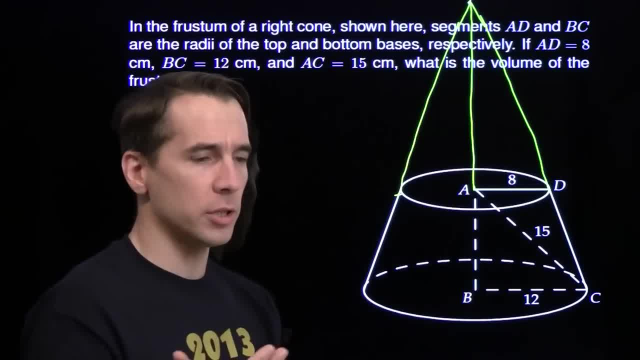 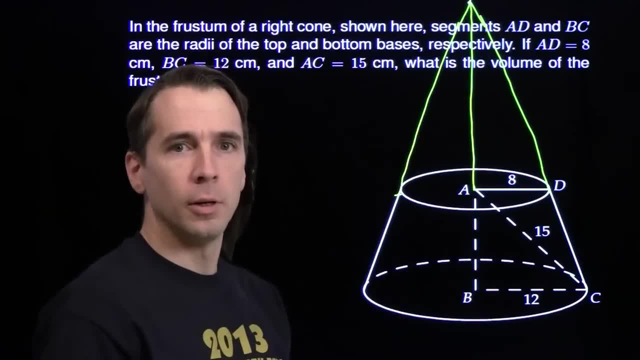 cone. So that means that what's left over is 27 minus 8 is 19.. This piece down here is 19 27ths of 2.. That's P the large cone. Well, now all I have to do is find the volume of the whole big cone and 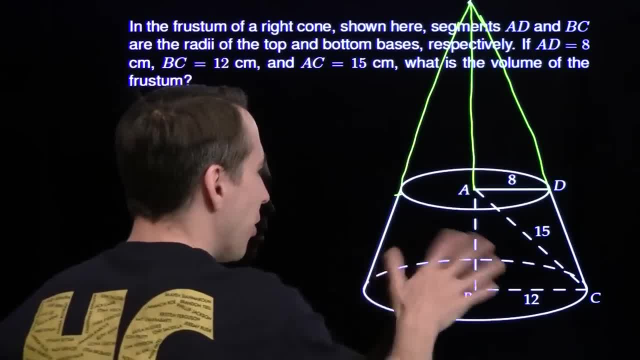 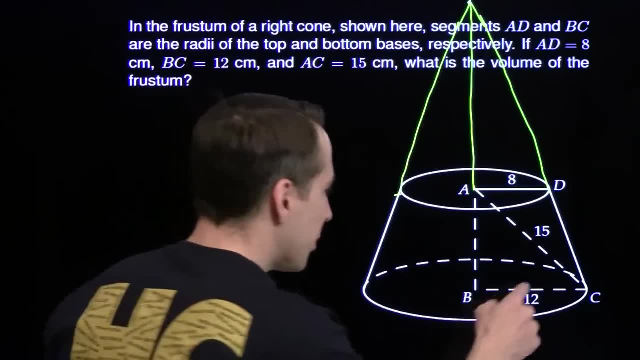 then take 19, twenty-sevenths of it and I can handle a cone. So I don't have to think about the frustum anymore. I've got the radius of the base of the cone. Now all I have to do is find the height. I've got this piece right here. This is 12,. this is 15, so this is 9. 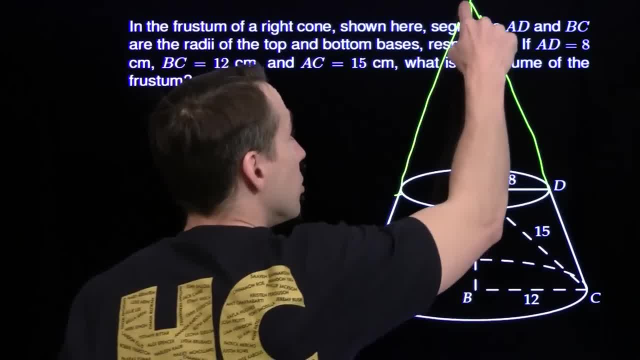 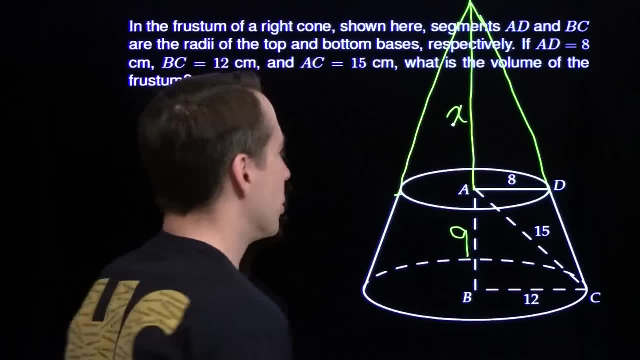 right there from the Pythagorean theorem of 3,, 4,, 5 right triangles, So to get the height of the whole large cone. all I have to do is figure this out, and that's a job for similar triangles. So you've got. this triangle is similar to this one, So we know that. let's. 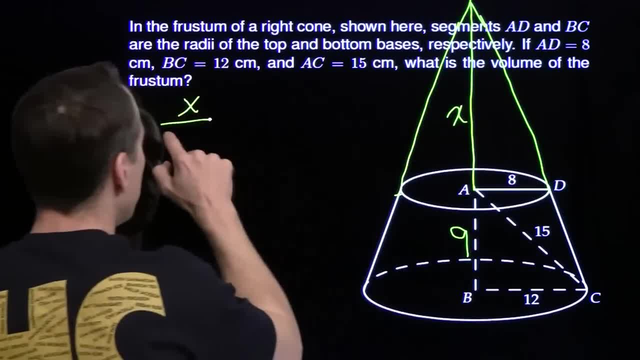 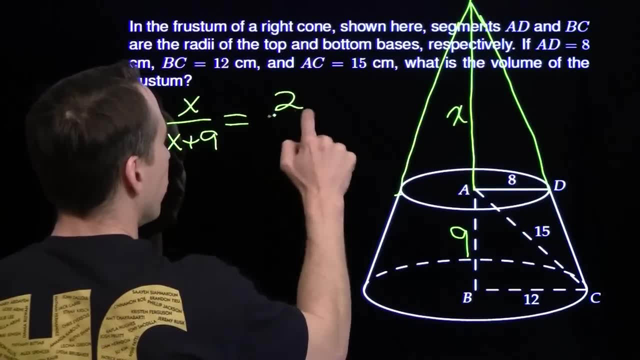 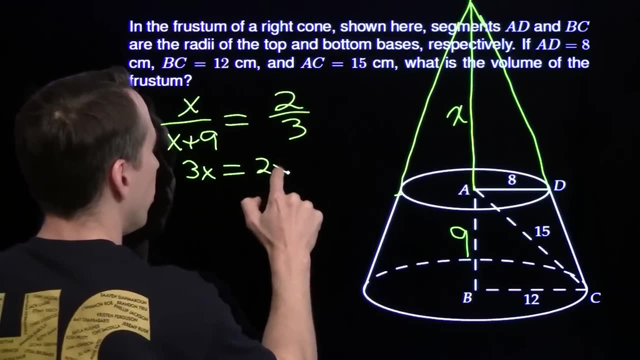 see, we've got x over. x plus 9 equals 8 to 12, which of course is just two-thirds. So I'll just multiply both sides by 3 and x plus 9.. We get 3x equals 2x plus 8.. So that's. 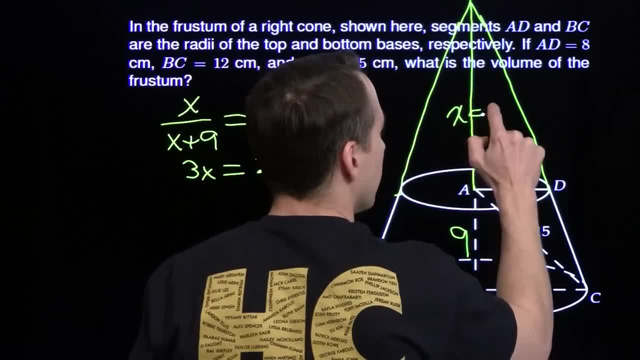 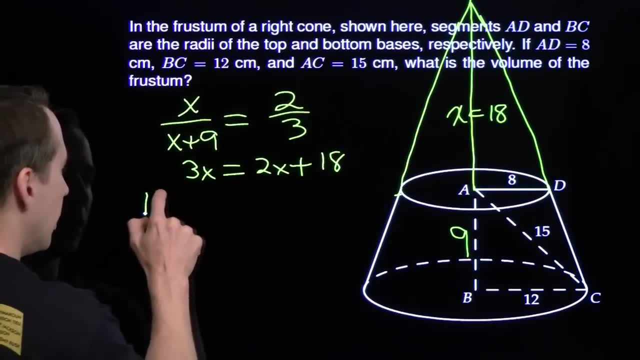 the whole thing 18, which tells us, of course, that x is 18.. And now I can find the volume of the whole large cone and the volume of our frustum down here is just 19, 27ths of the volume of the whole cone. so the volume of the whole 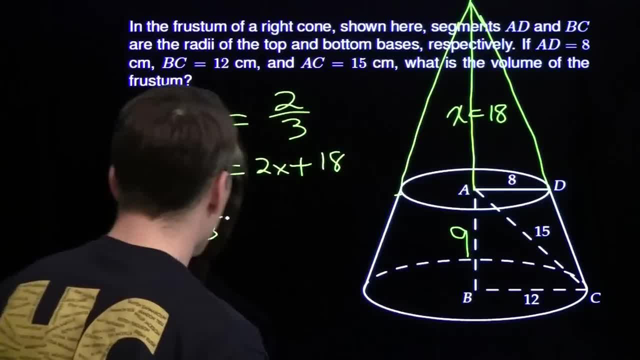 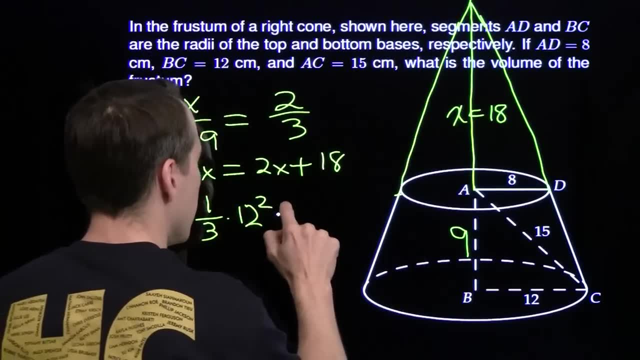 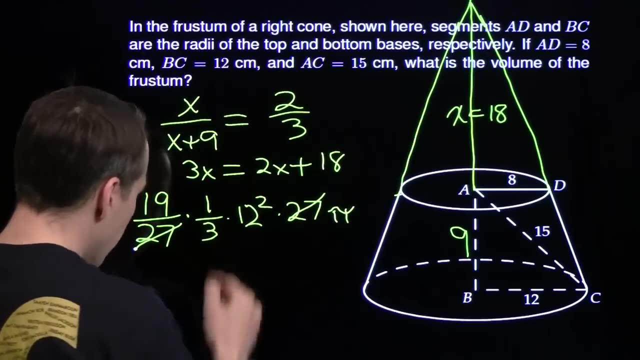 large cone is 1, 3rd times square of the radius, 12 squared times the whole height, which is 27 times pi. All right, so our 27ths. they cancel out Three cancels, so it knocks out part of one of the 12ths, so it leaves us with 4, oh boy.